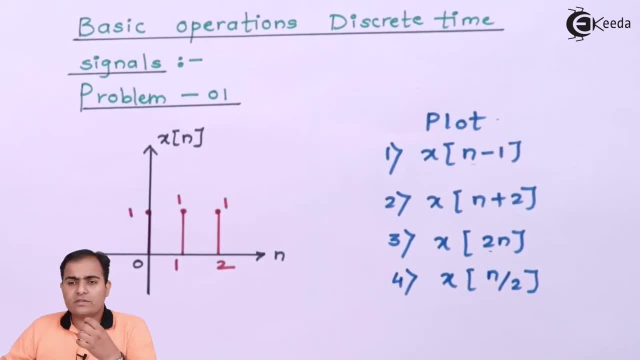 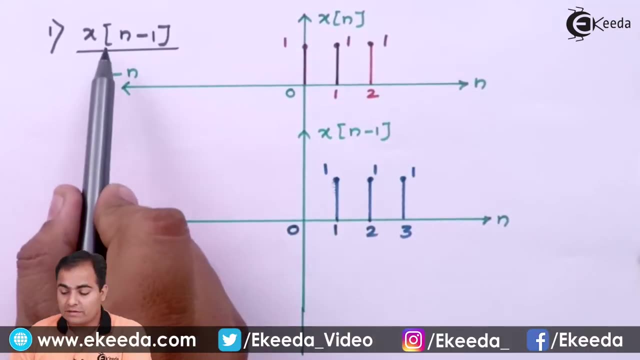 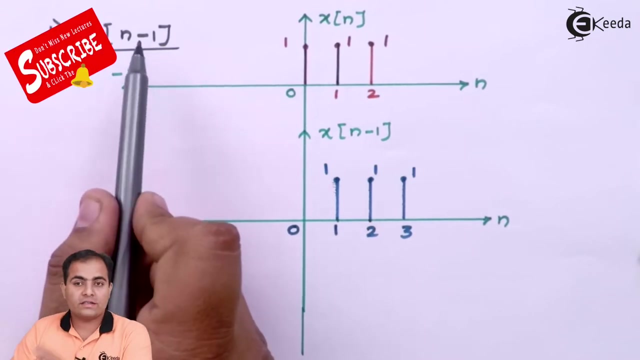 So we'll solve all the numericals one by one, how the solution will take place, how we are going to solve this numerical. well, let's see one by one. Now, the first part is x of n minus 1.. As I told you earlier, the minus sign means what. the graph will be shifted towards the right hand side by 1, or you can say the graph is delayed by 1.. 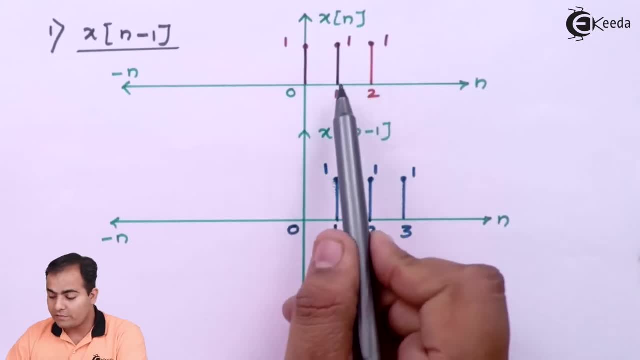 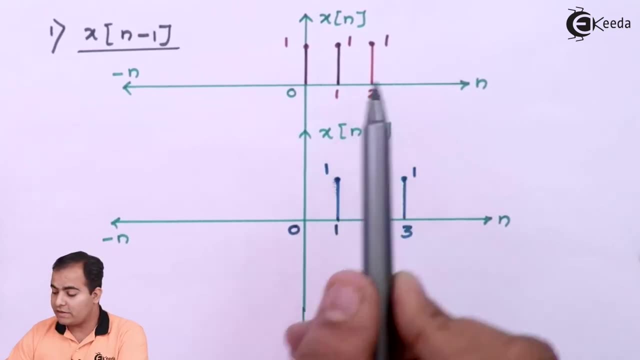 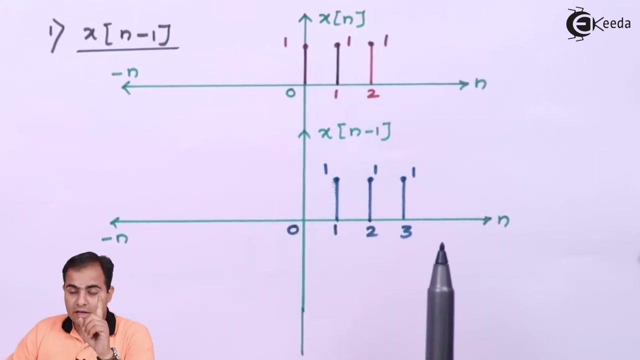 Now the original x of n sample sequence is already plotted. now, as I said, the graph is shifted toward right hand side by 1. means what? all this time scaling strengths will be shifted towards right hand side by 1. that is, 0 will be shifted on 1, 1 is shifted on 2 and 2 will be shifted on 3, but amplitudes will not be affected. amplitude will remain same, that is, at the 0 we have amplitude 1.. 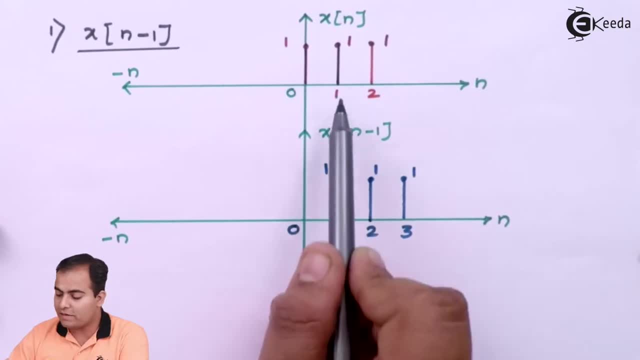 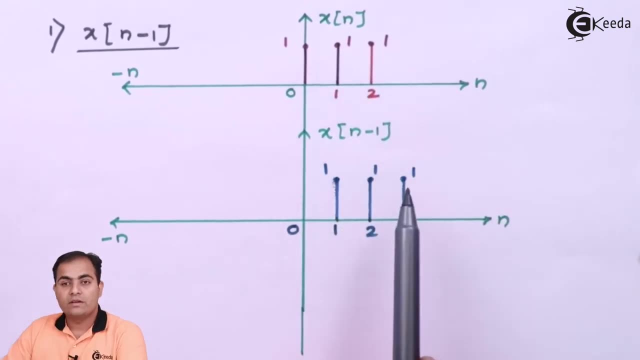 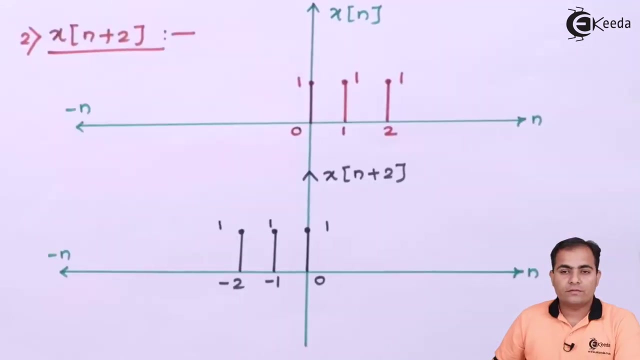 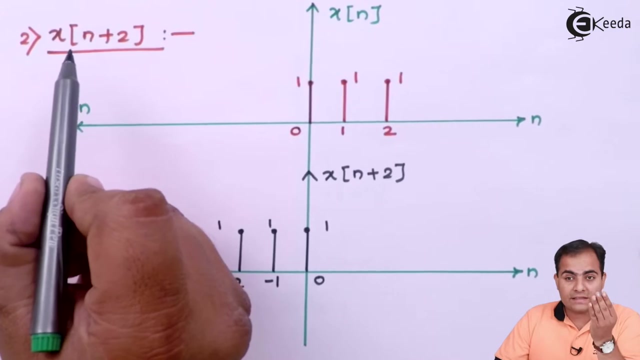 So, after Shifting, this point will be shifted at 1, having amplitude 1. similarly, in case of 1 and 2, both this point shifted on 2 and 3 respectively, where the amplitude remains same. this is how we are going to perform the time shifting property. now the sub part of this function that we will say you. now the second part of this function, the numerical, is x of n plus 2. n plus 2 means what plus sign mean, indicates or defines. we have to perform time advance operation. that is, your graph is shifted towards right hand side by 1.. 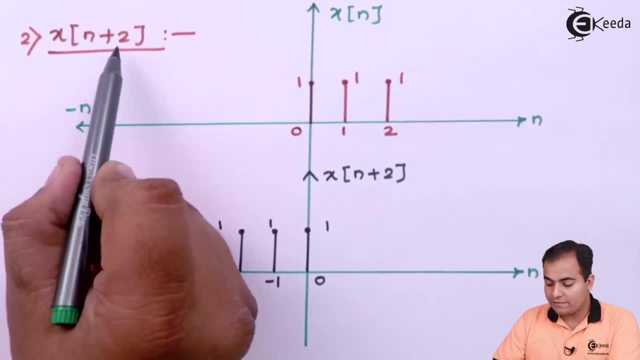 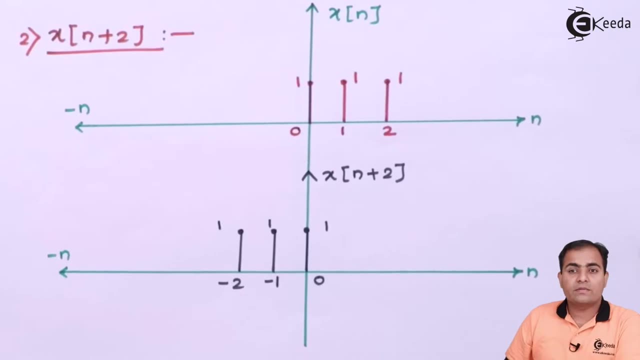 Half is shifted towards the left hand side. now by how much value? that value is already given and it is 2.. So all the time sync see sequences will be shifted towards the left hand side by 2. now how, let's see. Look at here. all the samplers already have exponent plotted here byまず present bunlar in such 0. when I do. 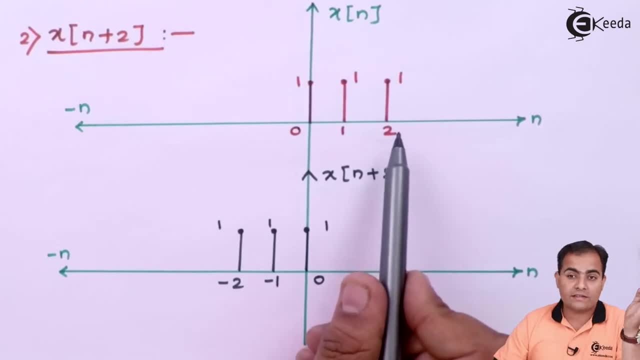 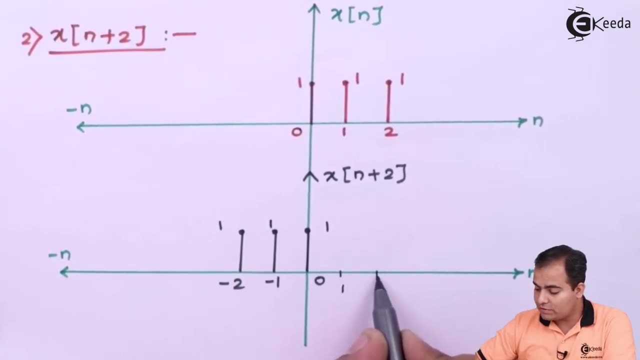 surface with Gerber too: 2. that is love how we can say that it is shifted by 2. so these are the original sequence. this sample will be shifted towards left hand side by 2. that is, this is first shift and this is second. 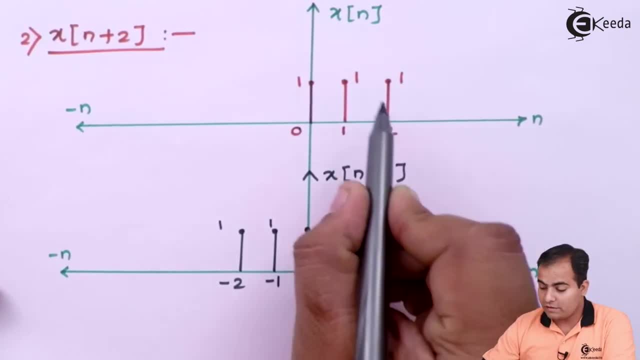 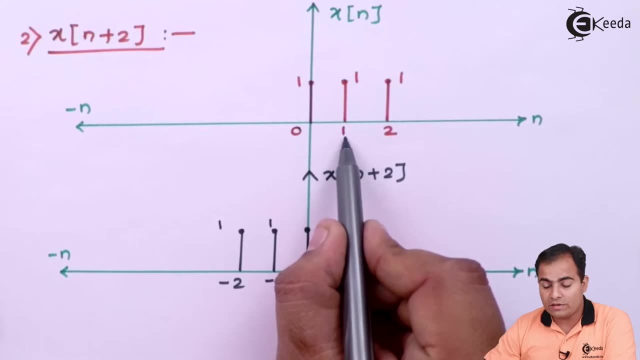 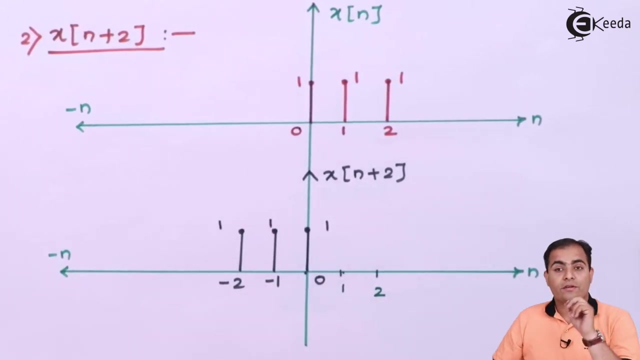 shift means this sample of x, of n, which is present on 2, now it is available at origin. similarly, sample which is present at 1 originally, now it is available at minus 1. now the sample which is present at 0, now it is available at minus 2, so we can say that all the instances. 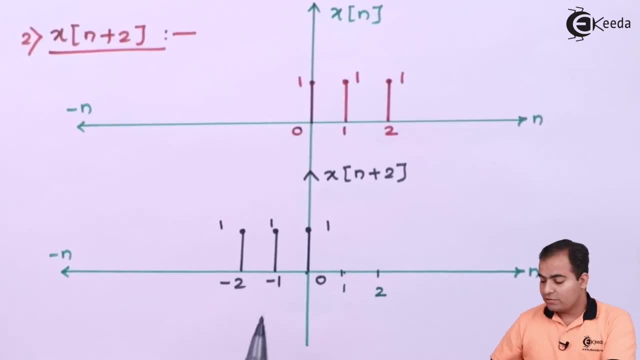 now shifted towards the left hand side by 2. so look at here: all the samples are shifted. amplitudes will not get affected because this operation is performed with respect to time only, not with the amplitude. so remember, only time instances will be shifted towards the left. 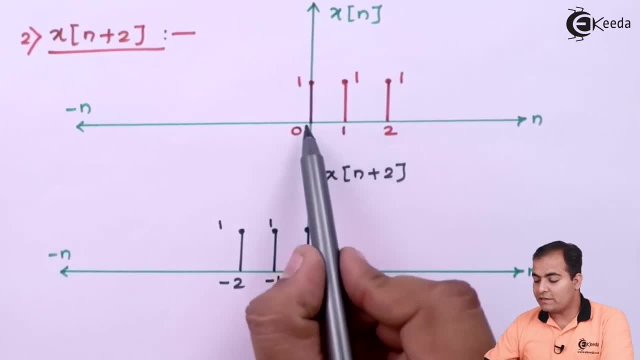 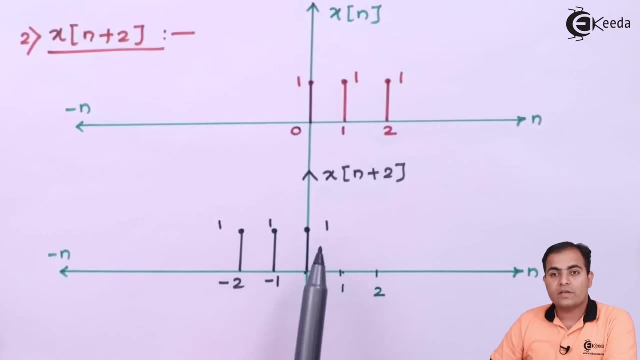 hand side and the amplitudes remains same. so you can see that at the 0, 1 and 2 we have amplitude 1, 1 and 1, 1 and 1, 1, and after shifting also the amplitude is same. now we will solve. we will study the third part of. 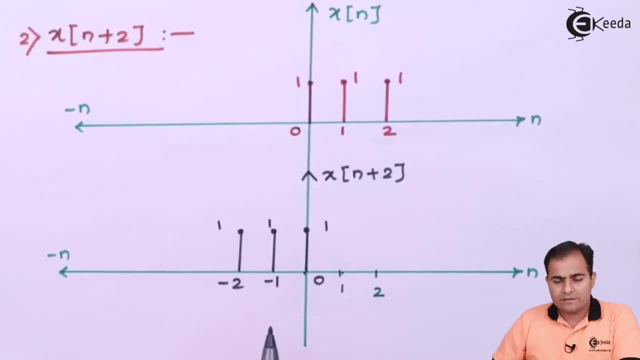 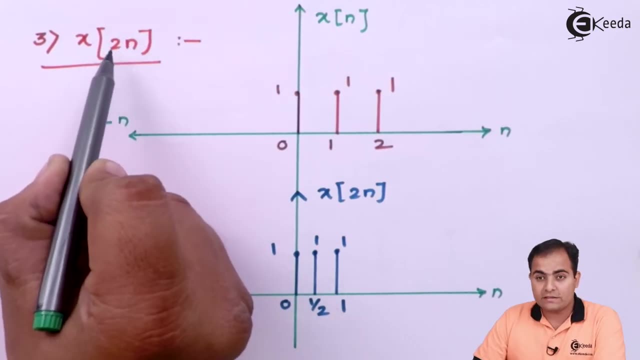 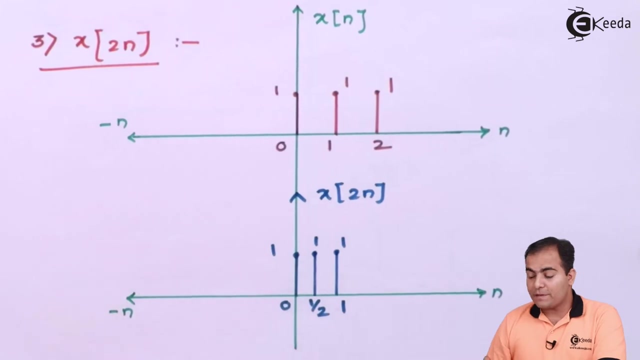 this question how the time scaling operation is can be done. let's see now in third case. here we are going to perform time scaling operations, but in this time scaling is divided into two parts: a compression, one. second one is expansion. now this is the part of a compression. 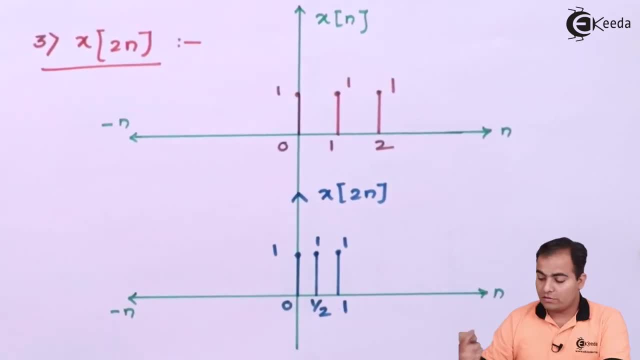 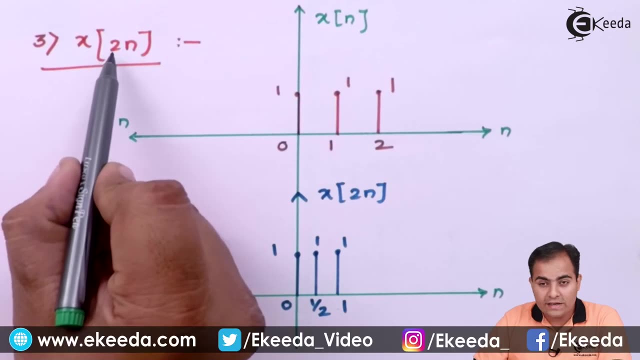 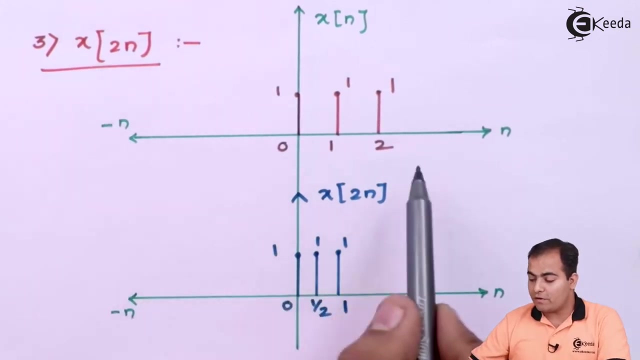 compression means all the time sequences will get shrink by value of two. this is the value of alpha, which is the scaling factor. now, it is if the scaling factor is present in multiplication form, and then what we are going to do is we are going to perform the division. all the samples will be. 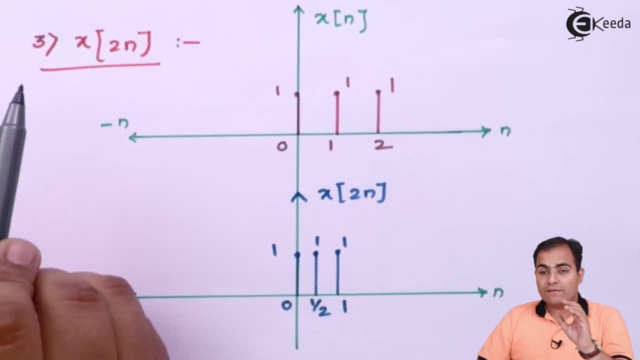 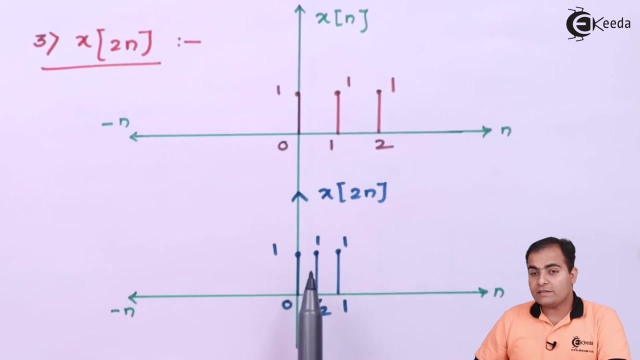 divided by given alpha value. if the alpha value is present in denominator or in fraction form, we always perform the multiplication. now let's see how this process is going to be performed. so, first of all, x of 2n. 2n means what the all the samples will be. 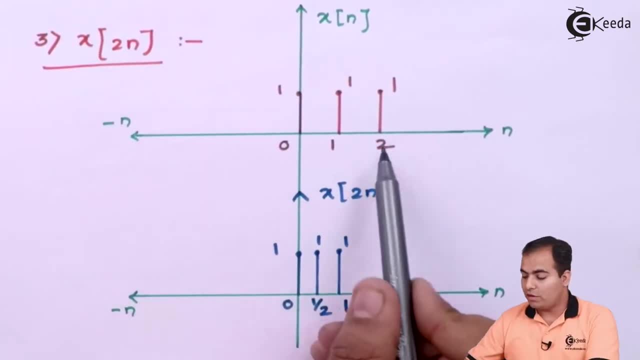 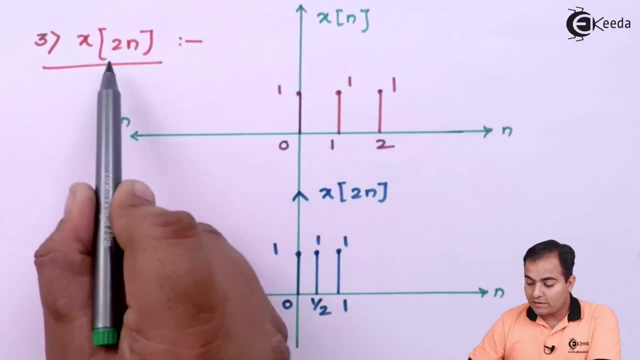 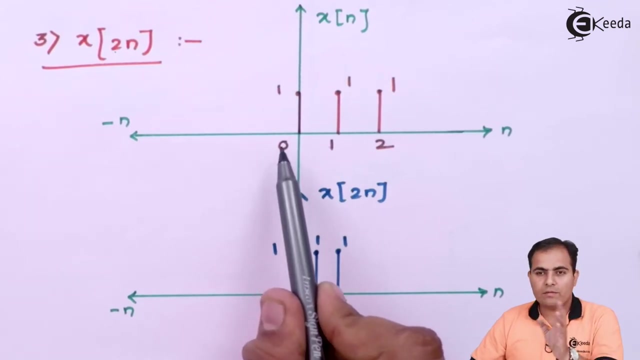 divided by given alpha factor, that is 2, so all the samples will be divided by 2. amplitude will not be affected, as i told you earlier. so if the alpha value is 2, so we'll divide all the samples by 2. so 0 by 2 remains 0, so these samples will not be changed. the location of this origin will remain. 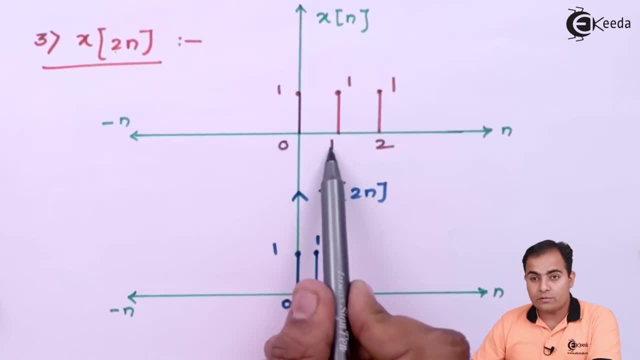 same, whereas if we divide 1 by 2, this location will be changed to half. that is now this first location now available at half. similarly, look at here: in case of 2: if we divide it by 2, the new location of this sample is 1. that is, 2 by 2 is 1, so it is available at 1. but look at the amplitude. the amplitude in x of n is: 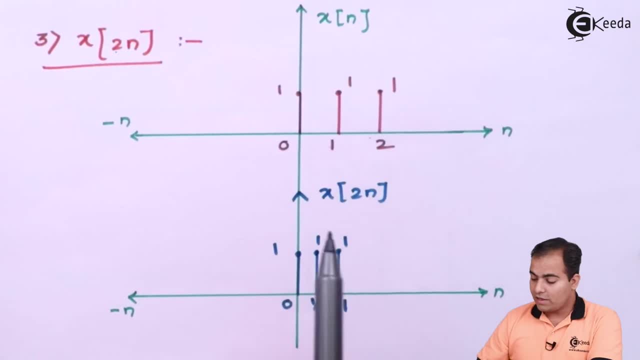 at 0, it is 1, 1 at 1 and at 2 it is 1. after performing time scaling, operation amplitudes will not get affected. so please remember now: this is how we are going to perform the compression operations now. the next part of this function is the numerical is expansion- how the expansion will take place. 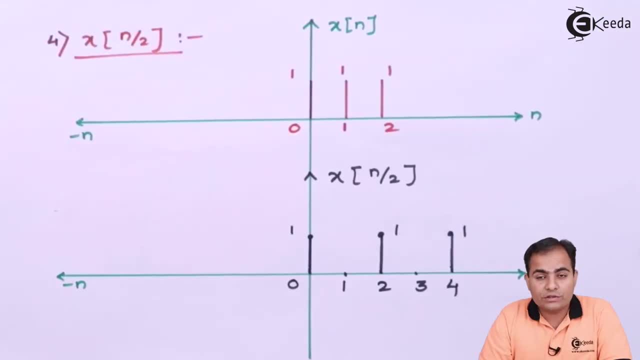 let's see 1 by 1. now. the fourth and last part of this power question is x of n by 2. as i told you earlier, if alpha value is greater than 1 means what we have to perform compression operation, and if alpha value is less than 1, mod of alpha value is less than 1. 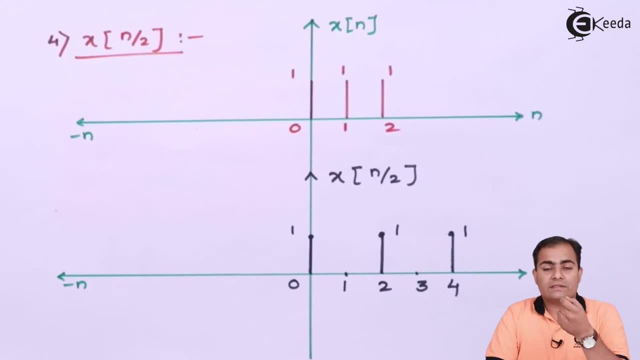 then we have to perform compression operation, or you can say that graph or signal get expanded. I will repeat: if alpha value is mod of alpha value is greater than 1, then we have to perform compression operation, or you can say that the graph will compress, will get compressed, or second: 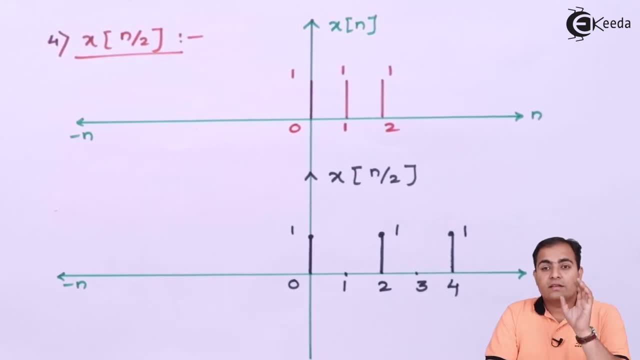 part is: if alpha value is less than 1, then the graph will be expanded or the time signal will get expanded by alpha. Now how the graph expansion and compression will take place, as I in the last previous numerical. the third part is: we have already discussed that is a compression. Now in 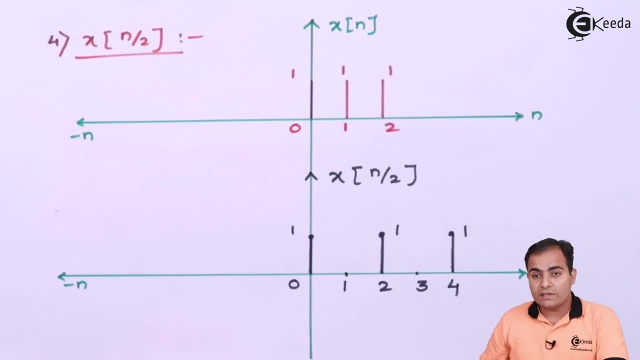 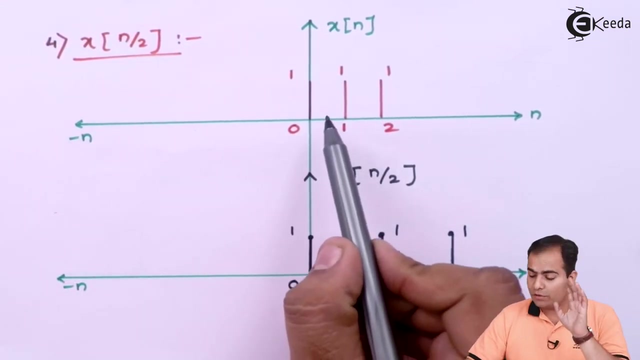 the fourth part, we are going to study the expansion. Let us see how the expansion is takes place Now. originally, x of n is already plotted. that is over here. Now, in case of x of n minus 2, this is the expansion operation x of n. that is original question original. 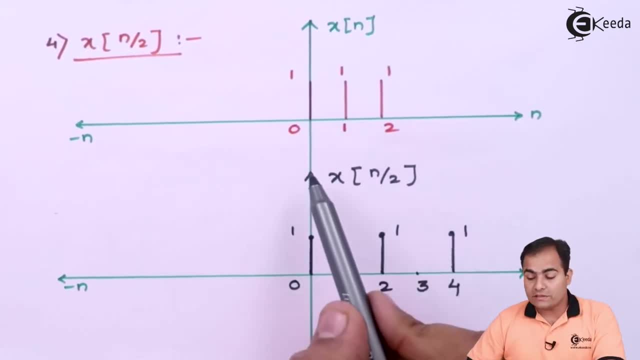 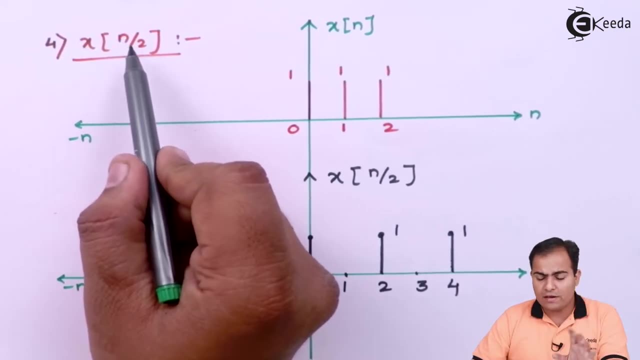 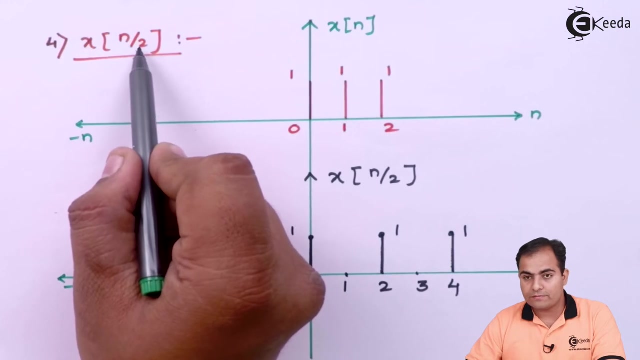 sample is already plotted Now how the expansion is takes place. as I told you earlier, if alpha value is less than 1, then just simply multiply that alpha value with each and every instant of time. Now, here, the alpha value is 0.5. so what you are going to do? 0.5 means it is 1 by half. 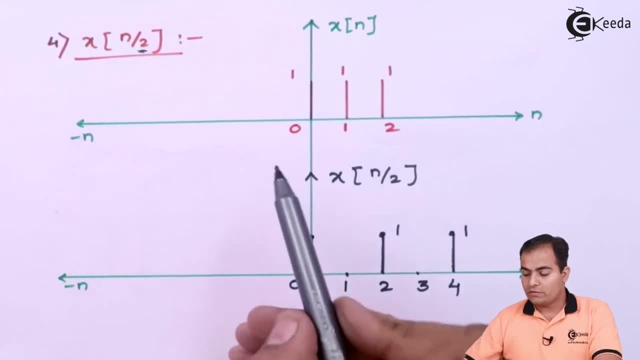 1 by half means this factor is important, which is a 2. So we will multiply all the time its instances by 2.. So 0 into 2 origin will not get affected, because the alpha factor, that is alpha is 2, is multiplied with the 0, answer is 0. So the amplitude remains.